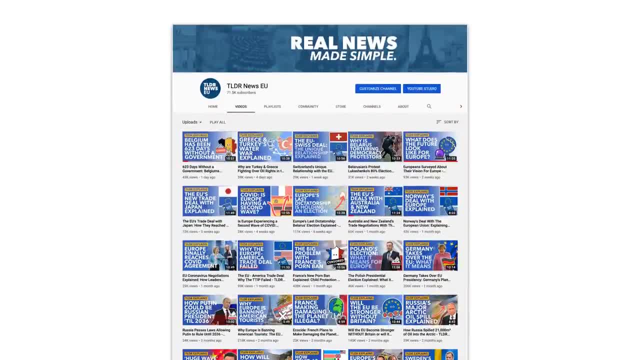 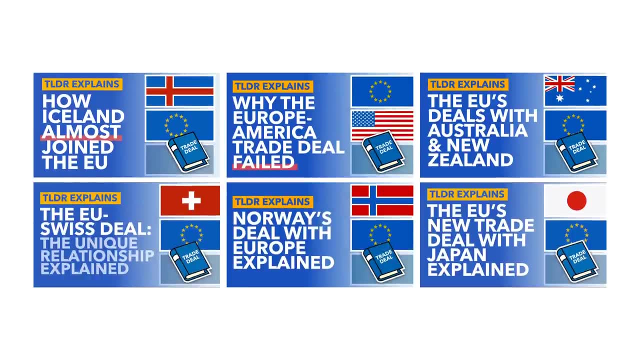 you are, then be sure to subscribe to the channel. We release a whole bunch of videos about the EU, including a series that we've linked down below about countries' relationships and deals with the Union. Anyway, TLDR EU is currently racing its sister channel, TLDR US, to 100,000 subscribers. 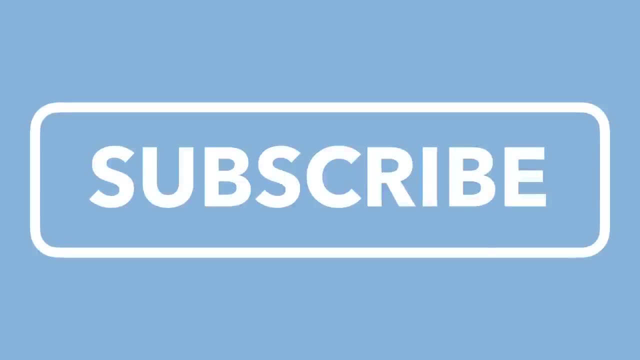 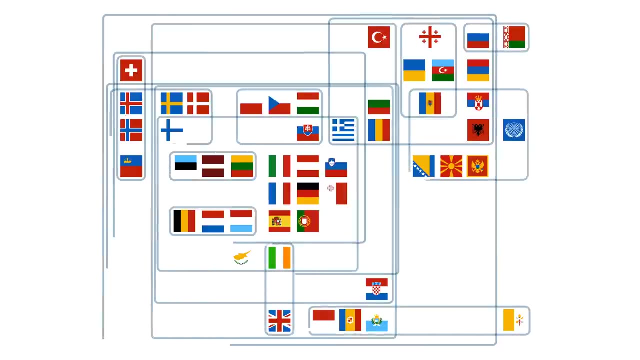 and while they have the lead, the EU is growing faster. So hit subscribe to make sure you see our future videos and lend us a hand. It goes without saying, really, that this map of EU relationships is complicated. I mean, look at it. The problem is that we want to keep this video under three hours long. 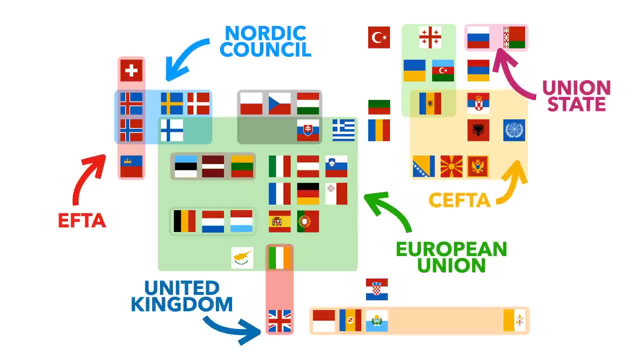 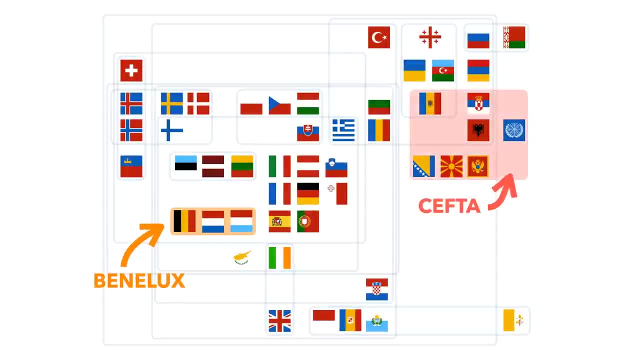 so we're going to be explaining the groupings pretty quickly, But if you'd like more details, then comment below, because we could do a whole series explaining groupings like Benelux, SIFTA and more. Anyway, let's start with the core of this diagram: the European Union. 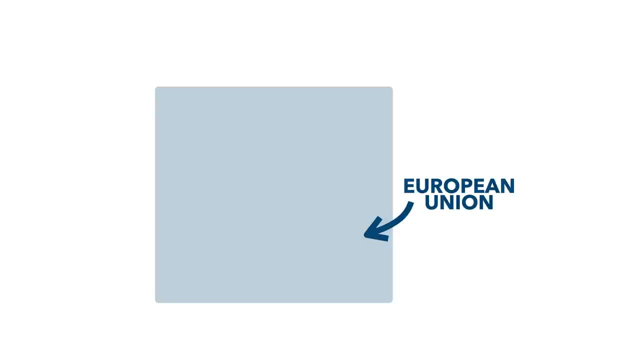 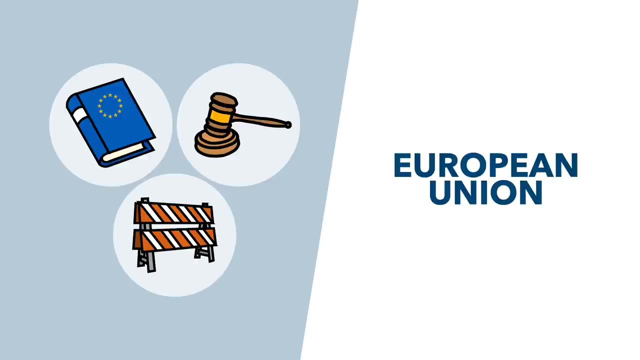 Hopefully this is pretty self-explanatory, but it's a political union currently comprising of 27 member states, formerly 28,. until you know, oh yeah, This truly is the core of the diagram, with these countries sharing laws, judicial oversight and sometimes even borders. 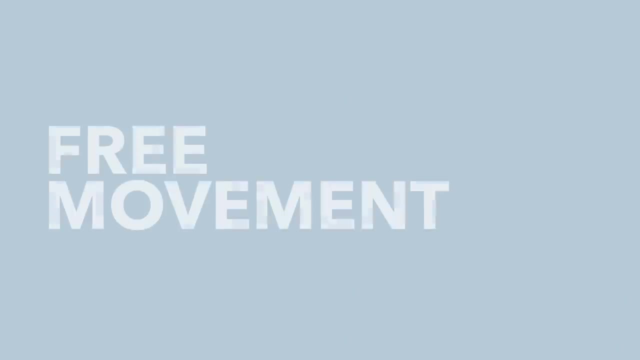 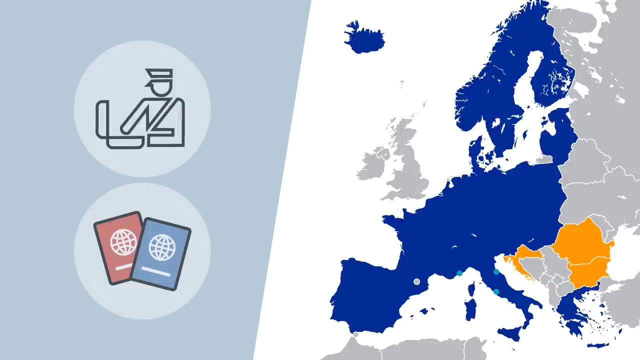 Speaking of borders, there's also the Schengen area. This is the area within Europe of the greatest free movement. Essentially, you can travel between these 26 European countries with no passports or border checks at all. Why just 26 and not the full 27 EU member states? 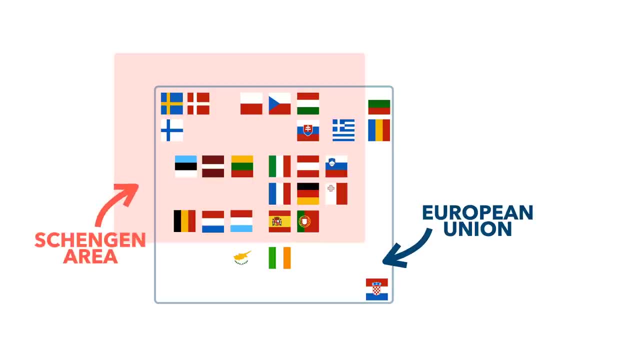 Well, firstly, you have to subtract Ireland, which, as an island nation, was able to secure an opt-out, something that the UK also had when they were a member. There are also another four EU countries who aren't part of Schengen: Bulgaria, Croatia, Cyprus and Romania. However, unlike Ireland, 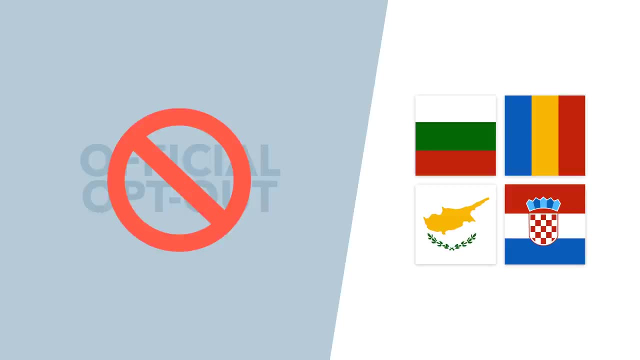 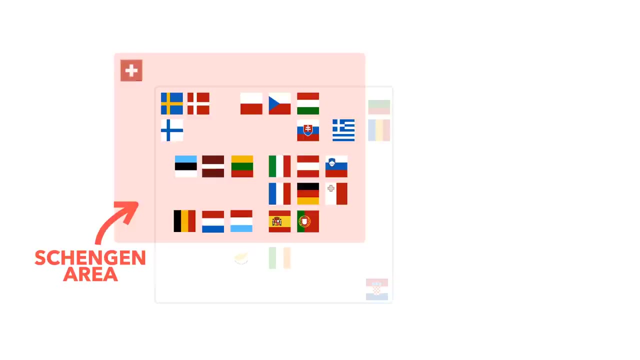 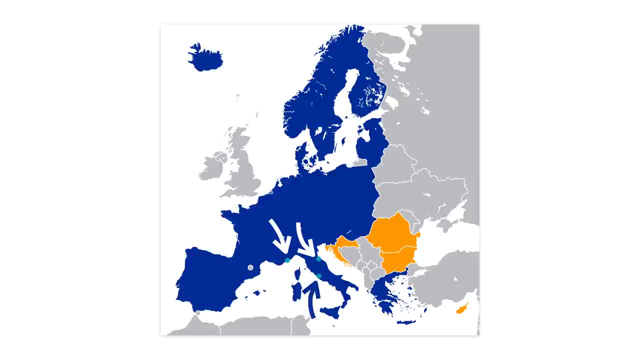 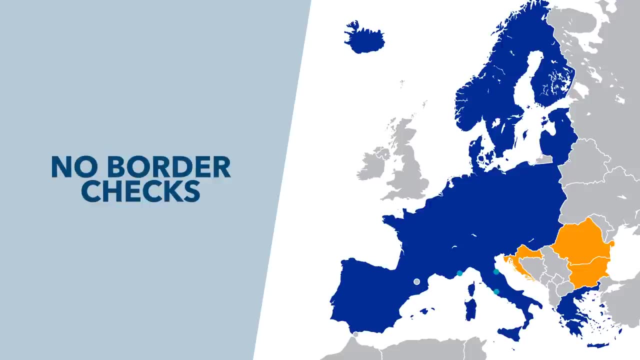 States. Monaco, San Marino and the Vatican City are also de facto members. They're not officially part of the agreement but in practice there are no border checks when entering or exiting the states. So in practice they kind of are part of Schengen. And remember I did warn you this was. 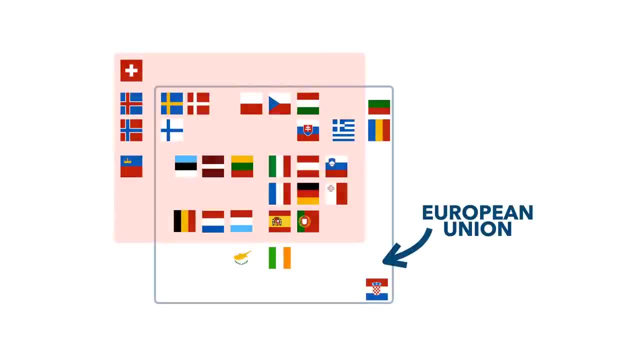 going to be complicated. Let's circle back to Switzerland, Iceland, Norway and Liechtenstein. They're in Schengen, but not in the EU, remember. However, they're also in the European Free Trade Association. We've covered EFTA a number of times before on this channel, but in its simplest terms. 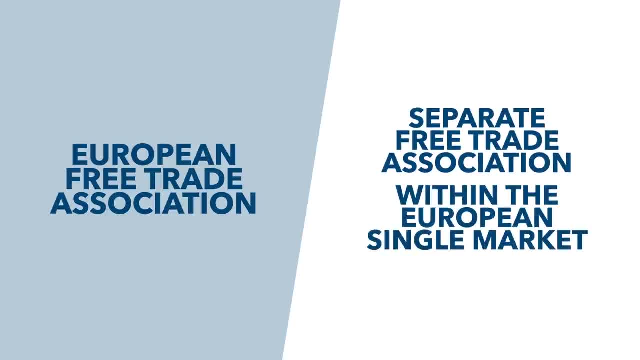 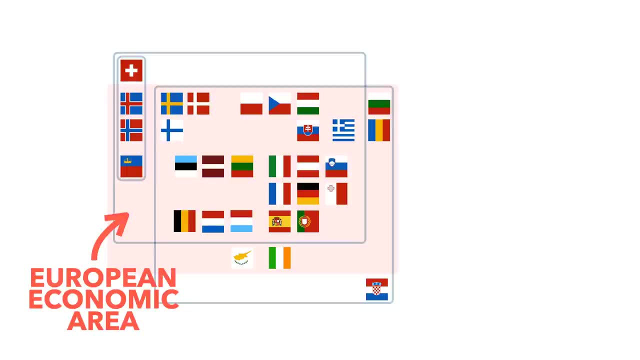 EFTA refers to a separate free trade area that participates in the European single market through the European Economic Area. Speaking of the EEA, in effect, it's the EU single market extended to allow access to EFTA members except Switzerland. Actually, Switzerland isn't the only. 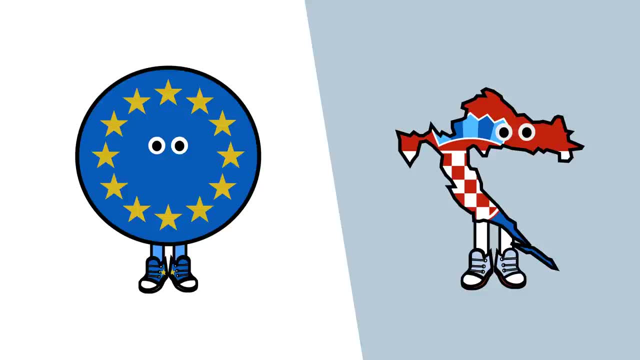 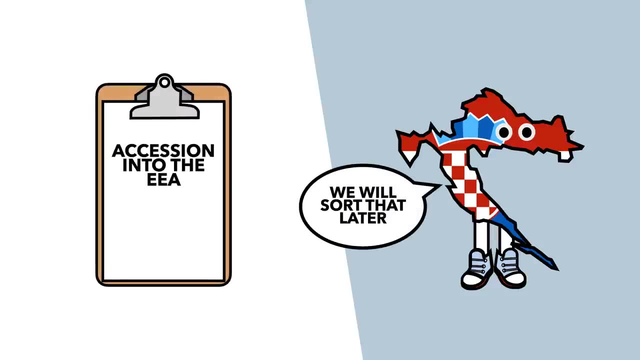 exception. Croatia is a member of the EU but isn't officially a member of the EEA. As the youngest member of the EU, it's the EU that has the most access to EFTA members, except Switzerland, Joining only in 2013,. the country hasn't finished its accession into the EEA, However. 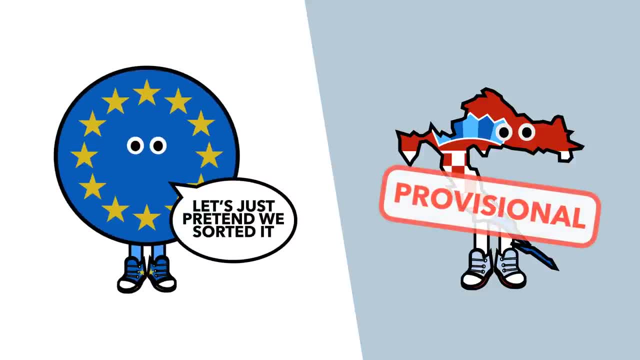 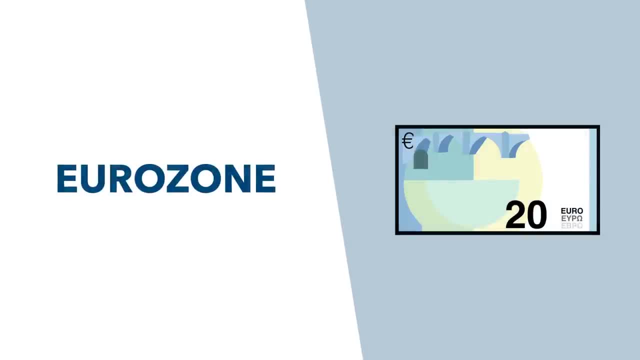 since April 2014,. they have provisionally been part of the area. Another grouping that scoops up a big chunk of the EU's member states is the Eurozone. As the name suggests, this is the monetary union of countries who use the euro as their currency. Critically. 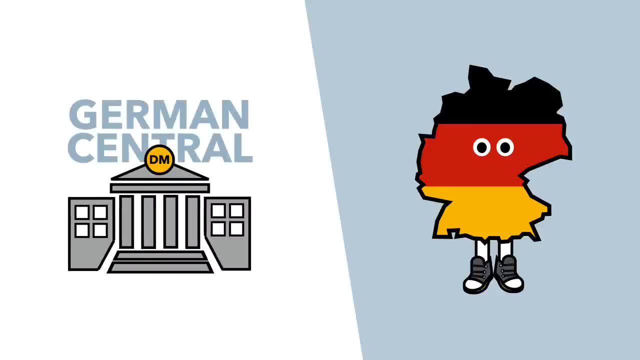 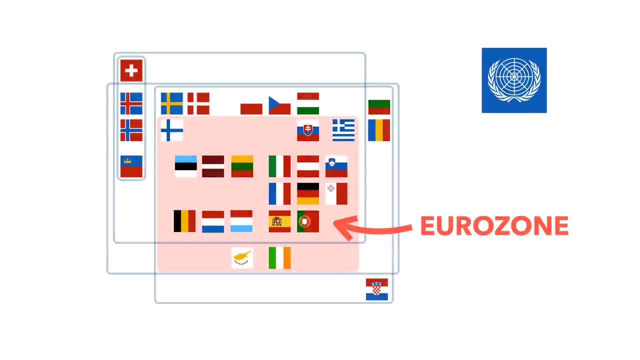 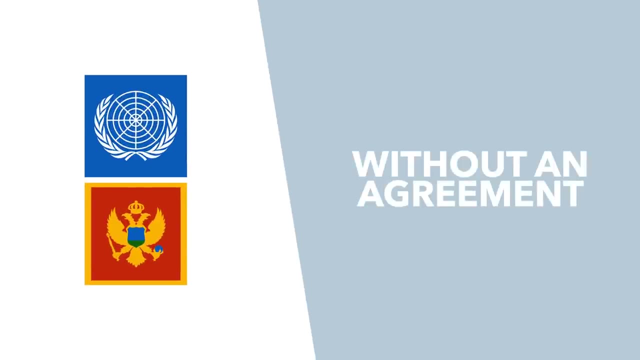 it's those who have abandoned any other currency, with their own central bank de facto replaced with the European central bank. Interestingly, by some definitions, Kosovo and Montenegro are also part of the Eurozone because they've adopted the euro as their currency. However, both did so without an agreement. 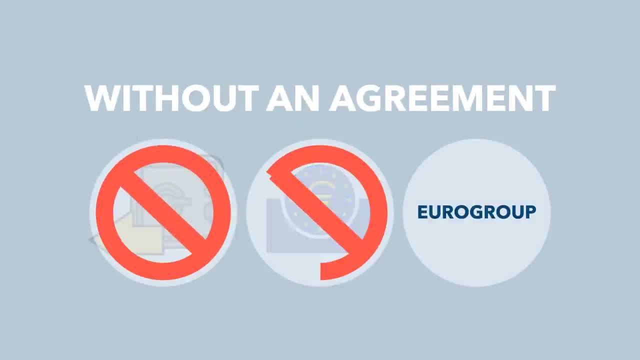 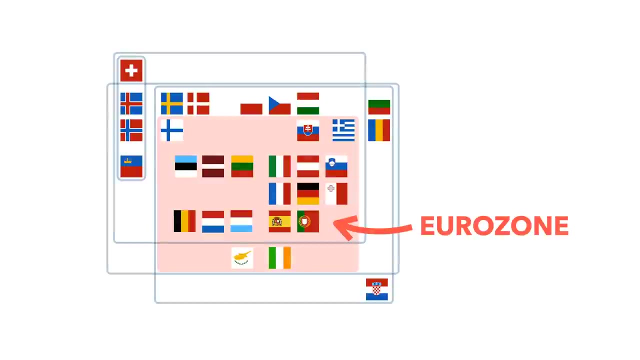 which means they don't have any issuing rights, any representation in the ECB or Eurogroup, or even a place on our diagram. Four countries have gone the official route, though, those being Monaco, Andorra, San Marino and- new entrant, the Vatican. These nations have 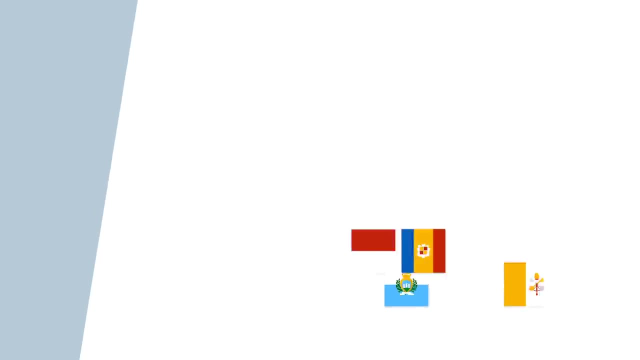 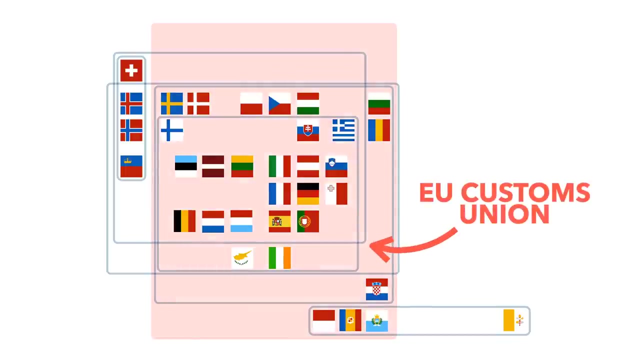 of their own accord, adopted the euro as their currency through a formal agreement with the European Union. There's one more really big one for us to sink our teeth into, and that's the EU's customs union, which is the EU's underlying trade bloc. This is the bloc which allows all member states to trade. 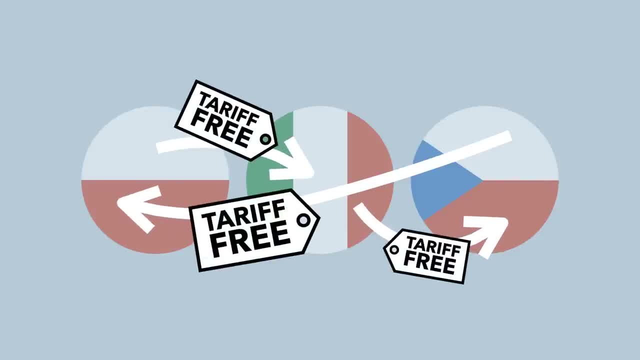 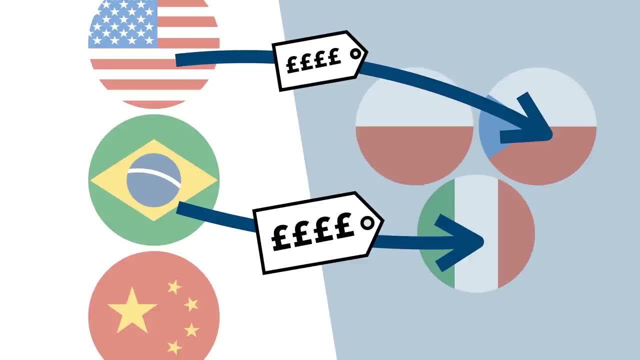 freely with each other without any tariffs in place, on the proviso that a common external tariff is enforced so that goods imported into the bloc, no matter which country they enter, are taxed appropriately. Essentially, members don't place tariffs on each other's goods and implement a standardised tariff on all goods being imported from outside. 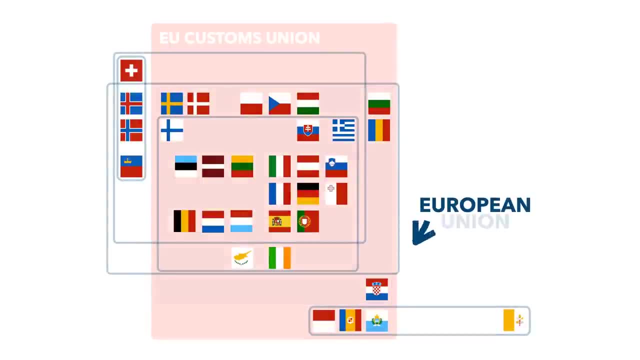 of the customs union. The customs union includes all 27 EU countries, but also includes a few others. Monaco and the United Kingdom are both full members of the customs union. well, Britain is, for now at least, and Andorra, San Marino and Turkey all have bilateral customs agreements with. 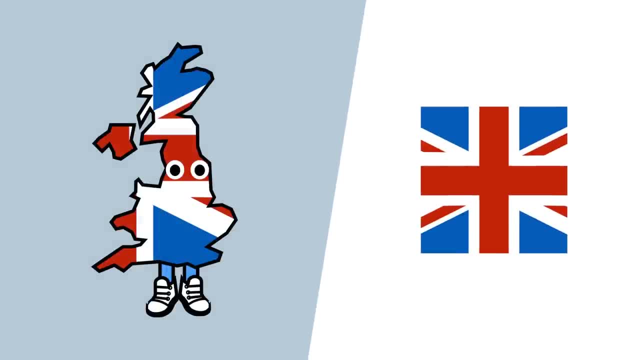 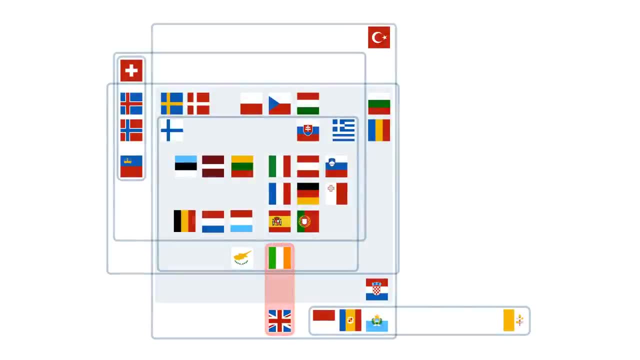 the EU, thus bringing them into the fold. Speaking of the United Kingdom, let's briefly talk about the other grouping the UK falls into. The United Kingdom is the only EU country in the EU, the one tying the UK to the Republic of Ireland. This isn't actually anything to do with. 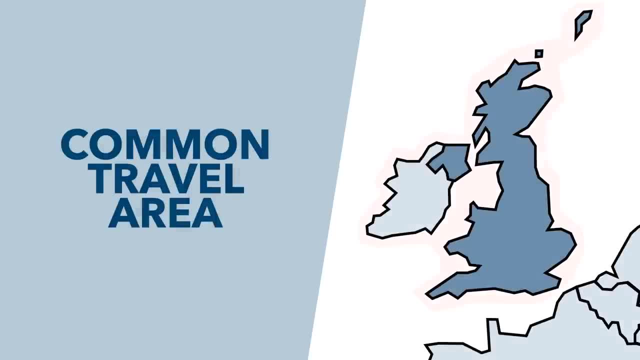 the EU, but instead is a free travel zone between the Republic of Ireland and the United Kingdom, including the likes of the Isle of Man and the Channel Islands. This allows for free movement between the two without any passport checks, Despite not being anything to do with the EU. 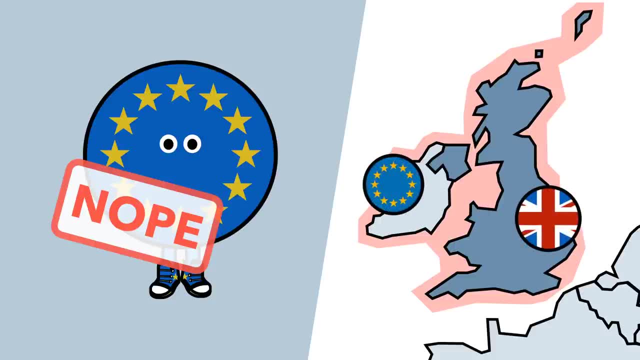 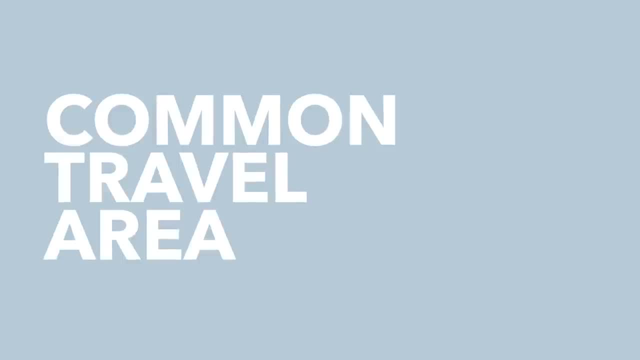 though, if the UK leaves the EU's customs union, this agreement could become more problematic, with one side in and the other out of the EU. Critically, though, this agreement pre-dates both countries' membership of the European Union by a significant time. Now I know I said the customs union was the last big one. 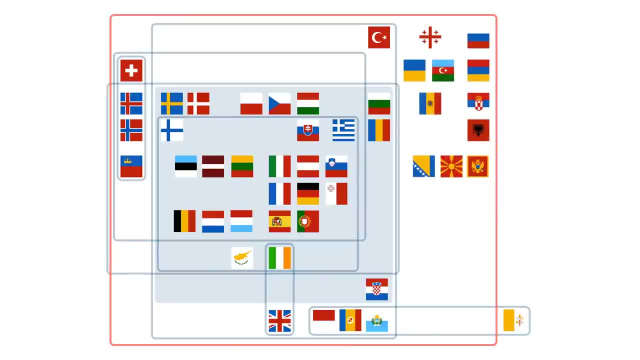 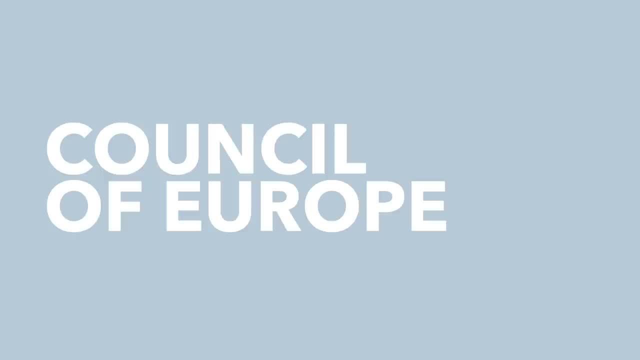 but there's actually one even bigger one than all of these: the Council of Europe. The Council of Europe, formed in 1949 following World War II, has 47 member states and is an international organisation which aims to uphold human rights democracy. 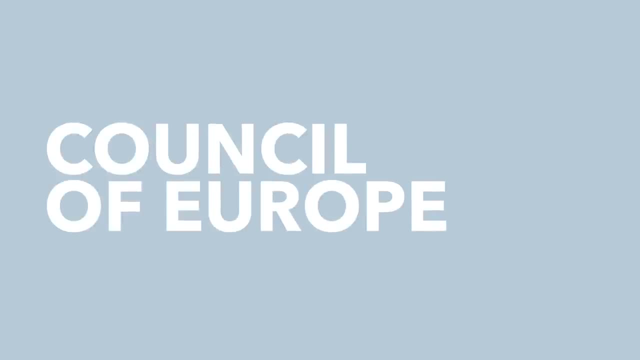 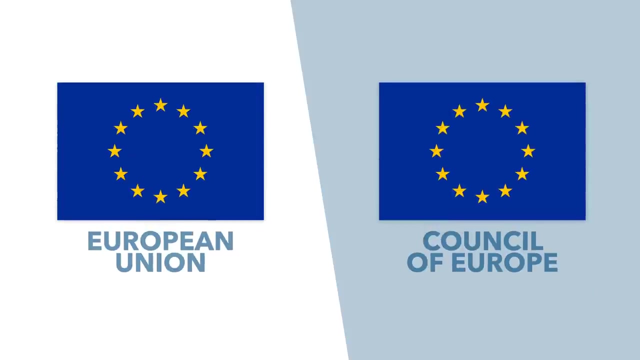 and the rule of law in Europe. Now, maybe this is a topic for another day, because it might be easy to confuse the EU with the Council of Europe, something that's not made easier by the fact they both have the same flag, which is again incorporated into the Council's logo. 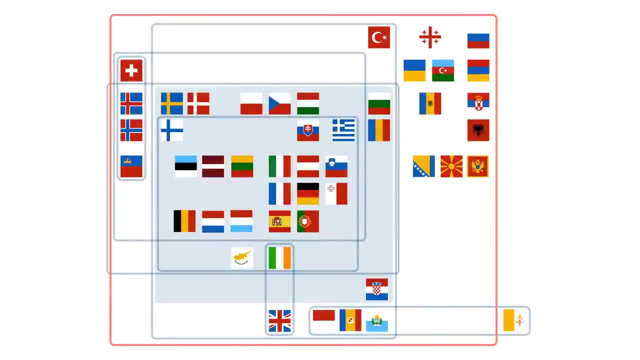 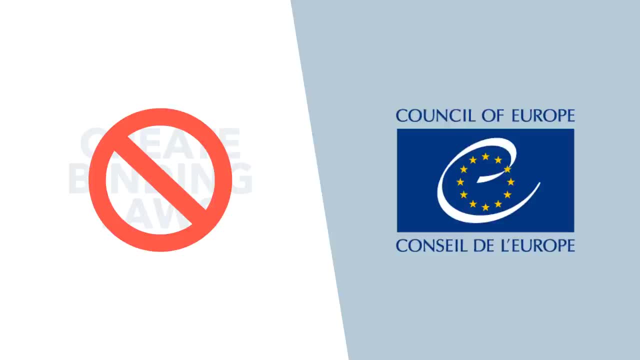 Very basically, the Council of Europe is a much larger grouping of countries, but it has much more limited powers. For example, the Council isn't able to create any binding laws. If you have heard of the Council before, though it's likely in relation to the 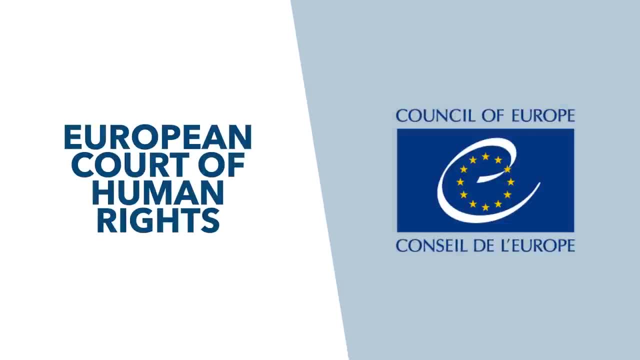 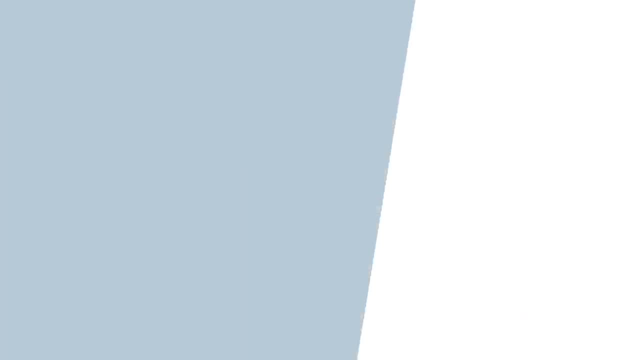 European Court of Human Rights, the institution responsible for enforcing the European Convention on Human Rights. So that brings our total flags up to 48.. Let's get to a nice round 50, and then do a quickfire round, Deal, Deal. 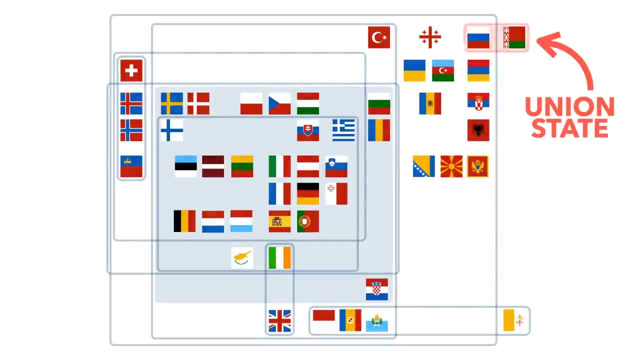 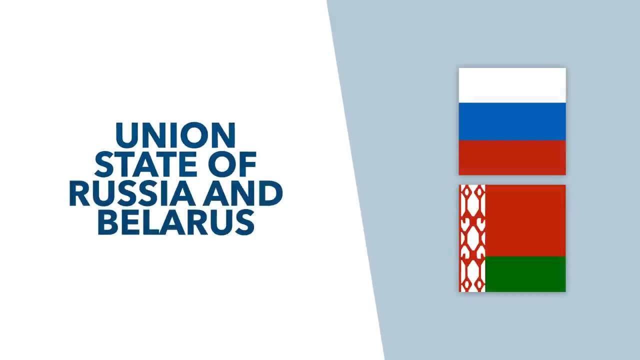 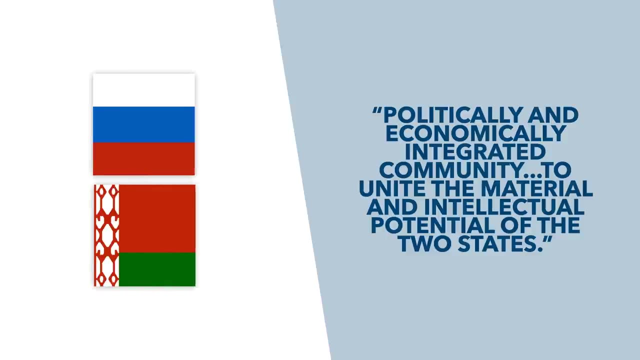 So Belarus enters the diagram thanks to its connection to Russia via the Union State, Often referred to by its full name, the Union State of Russia and Belarus is an international organisation with the aim of creating a politically and economically integrated community to unite the material and intellectual potential of Belarus. 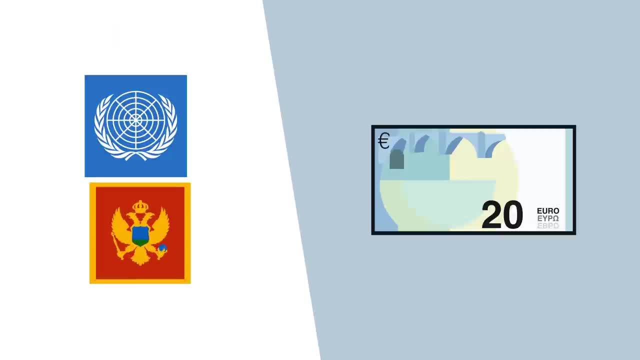 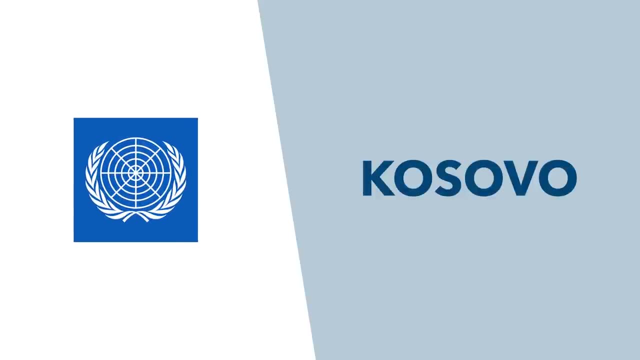 Finally, we mentioned them earlier, but despite adopting the Euro without an agreement, they've not made it onto the diagram until now. Kosovo Or- and this really is a story for another day- the United Nations Interim Administration Mission in Kosovo, who are brought into the 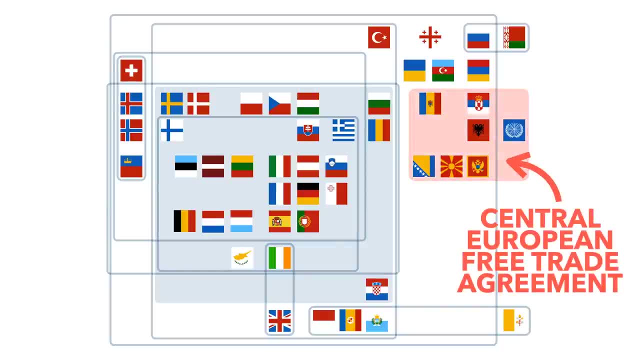 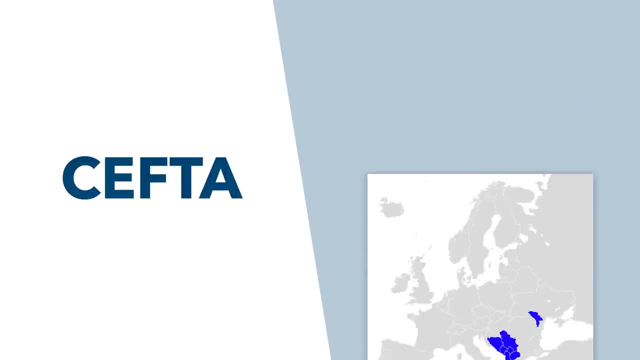 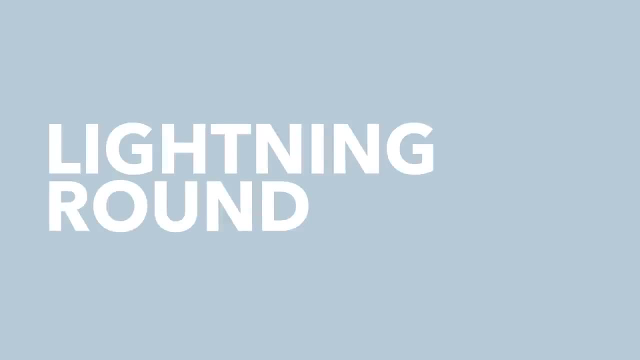 diagram thanks to their membership of the Central European Free Trade Agreement. As the name suggests, SIFTA is a free trade agreement comprising of a number of European countries that, misleadingly, aren't actually in the centre of Europe. So that's all 50 countries. You still ready for a lightning round to really clutter up this? 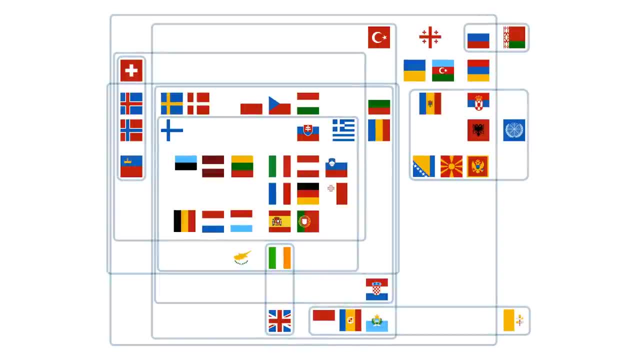 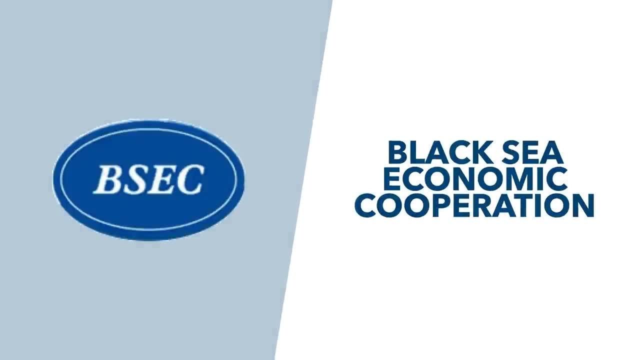 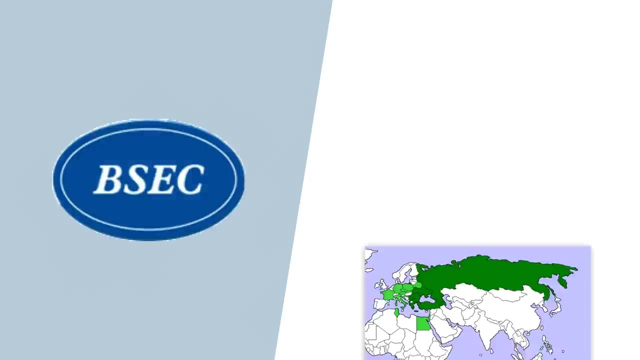 diagram Good. First, let's loop back to these countries and connect them with EU members via the Organisation of the Black Sea Economic Cooperation. They're self-described as a unique and promising model of multilateral political and economic initiative consisting of the countries: 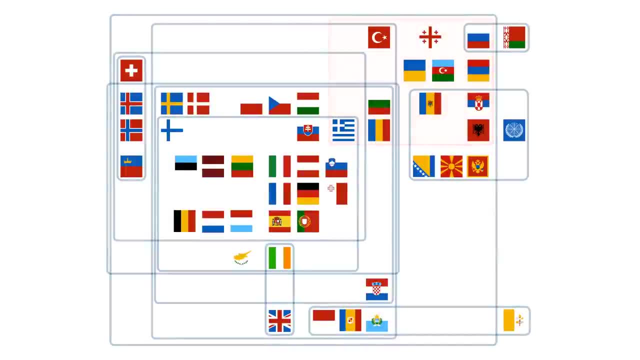 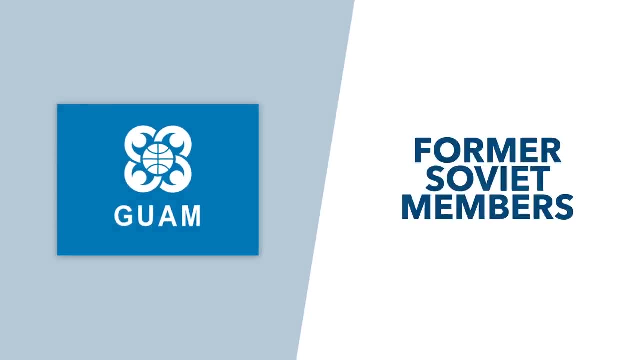 in and around the Black Sea. Within that grouping you've also got the Guam Organisation for Democracy and Economic Development. Guam gets its name from its member states, the four former Soviet states of Georgia, Ukraine, Azerbaijan and Moldova. Guam's main goals are strengthening democratic 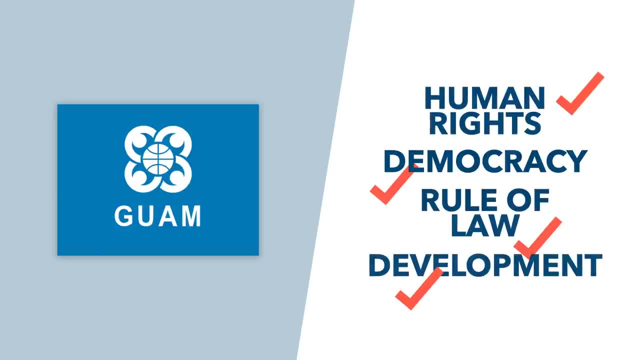 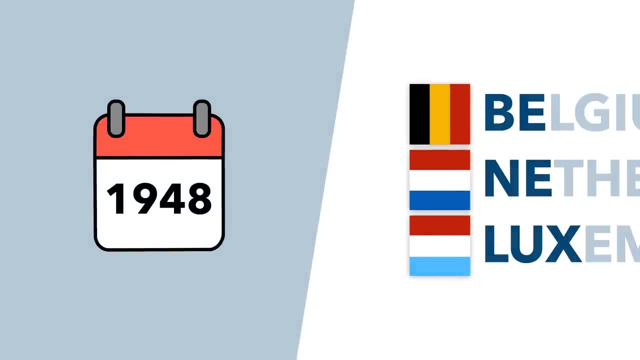 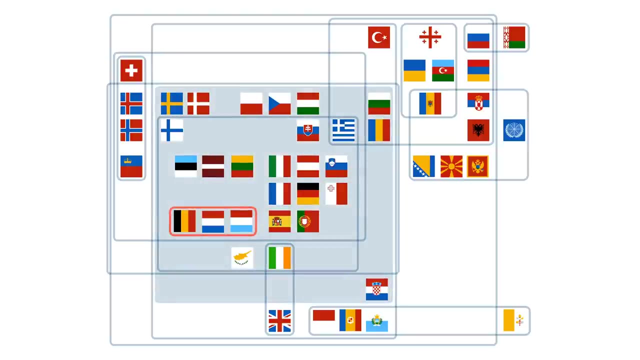 values, the rule of law, human rights, development and so on and so forth. Another group named after their founders, Benelux, first referred to a customs union established back in 1948. But today, given each country's membership of the European Union, Benelux tends to refer to the generic. 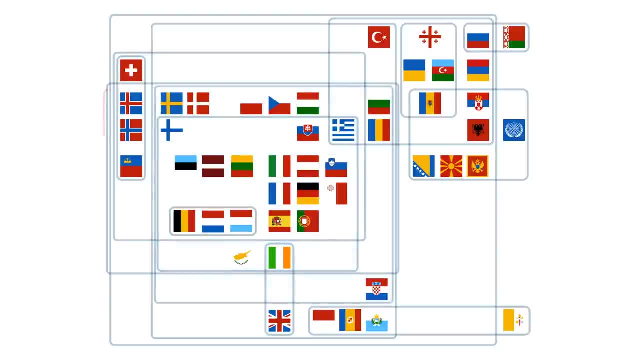 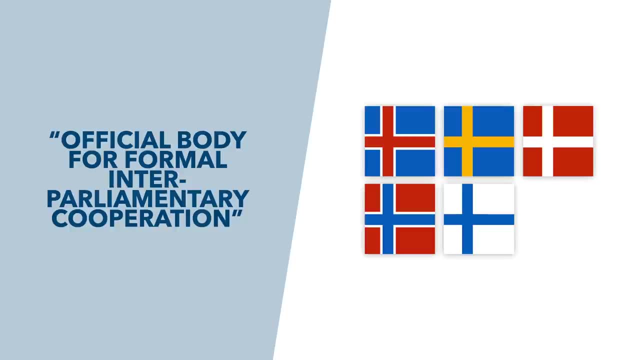 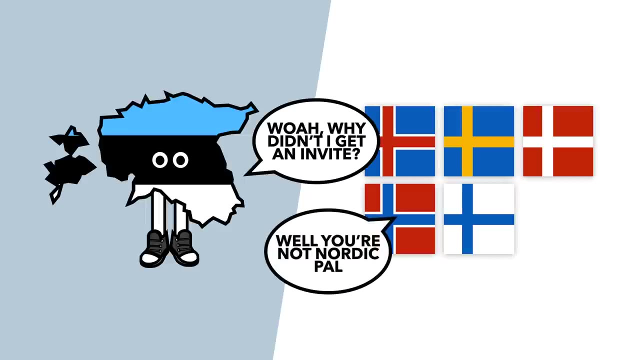 grouping of these three countries. The Nordic Council is combined of the Nordic states and describe themselves as the official body for formal inter-parliamentary cooperation with representatives from the Nordic countries. Just don't tell Estonia: they've been left out of this group because, despite not being officially recognised as Nordic by the international, 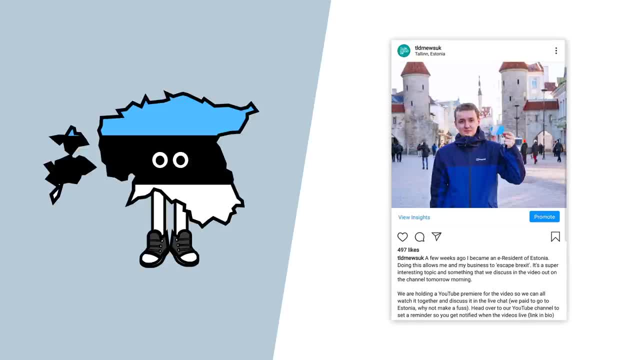 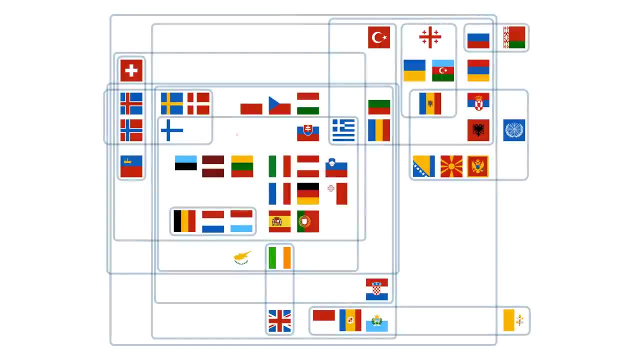 community. we were told when visiting that it's common for citizens to identify with their neighbouring Nordics. There's even a Wikipedia page about it. Two more, and this will be looking perfectly cluttered. The Visegrad Group, also known as the Visegrad Four, are an alliance of four central European 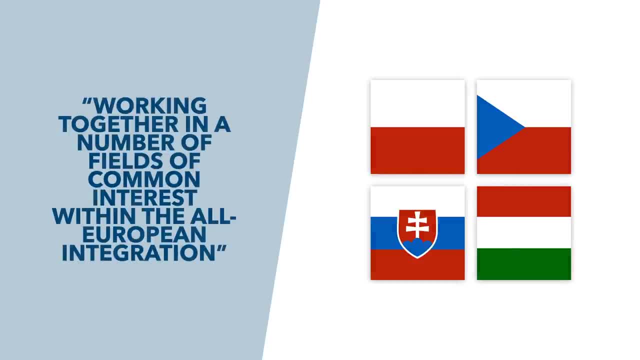 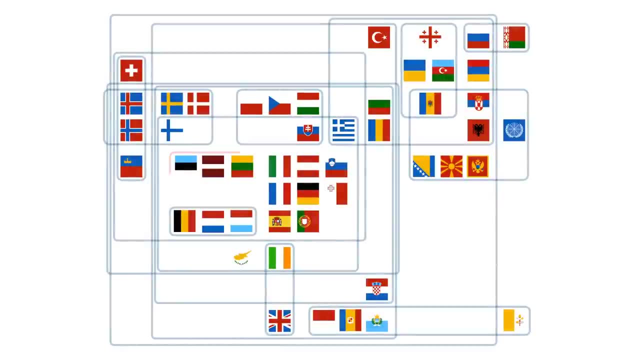 countries with the core aim of working together in a number of fields of common interest within the all-European integration. I did say that we were covering these quickly. Finally, we have the Baltic Group, who describe themselves as an international organisation for cooperation among 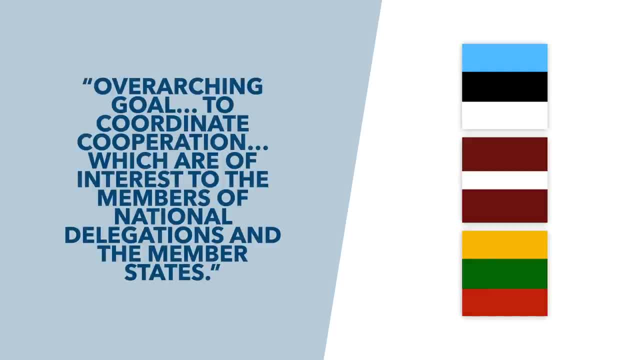 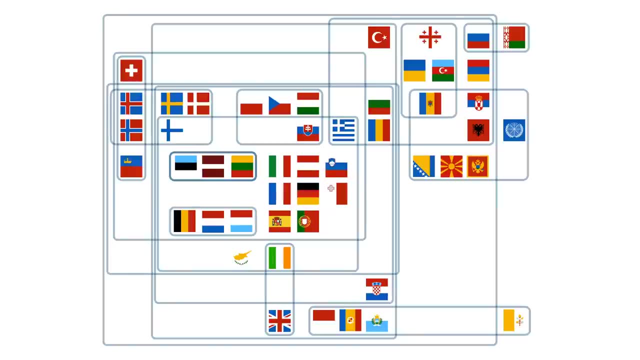 parliaments with an overarching goal: to coordinate cooperation which are of interest to the members of our national delegations and the member states. The Baltic Group is a group of member states that have been working together for a long period of time with the goal of 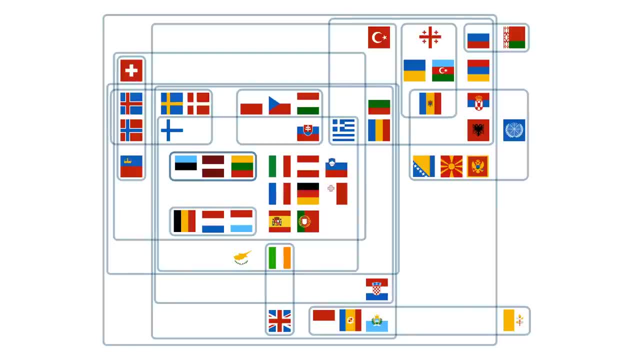 working together for a long period of time, with the goal of working together for a long period of time, and that's how all of these broadly European countries are linked together. What's the purpose of this diagram and of this video? Well, maybe it's to demonstrate the 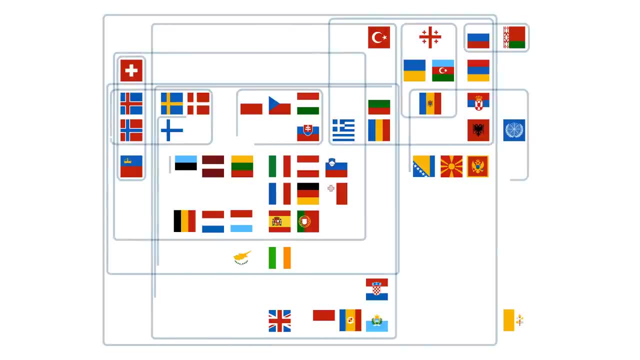 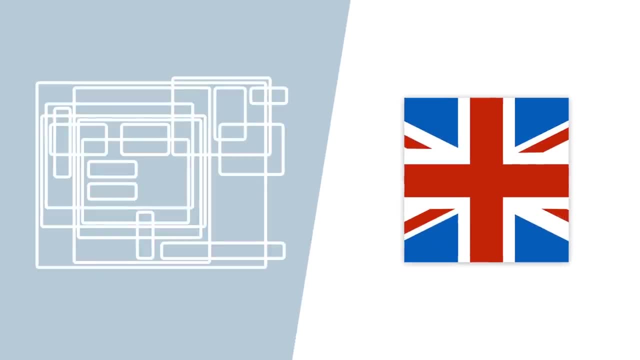 complicated array of groupings and agreements which exist on the continent of Europe. Maybe it's to illustrate the difficult, tangled world that Britain will find itself in having left the EU, Or maybe it was just an excuse to annoy the Estonians. Actually, scratch that last one, I like. Estonia, and we had a lovely time when we visited, Which is a nice thing to do if you want to get a bit of a taste of what it's like to be a part of the European Union. So that's our finished diagram, and 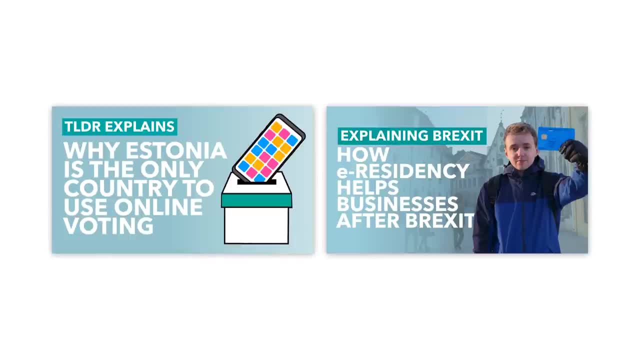 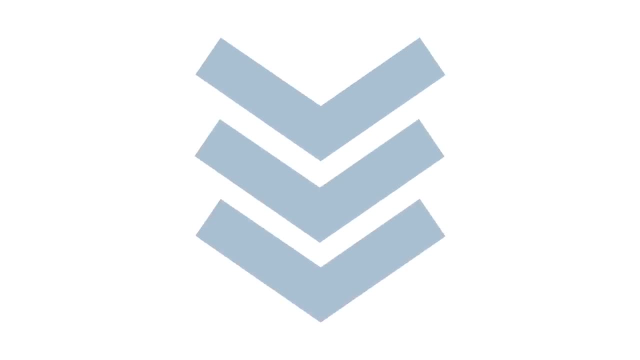 we visited, Which is a nice excuse to promote the videos we made about their e-residency scheme and online voting system when we visited Tallinn. Anyway, those videos are, of course, linked down below. Be sure to subscribe to the channel and hit the bell icon to be notified whenever we 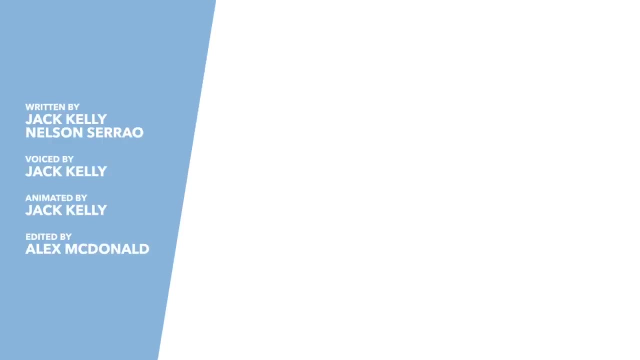 release further videos. Special thanks to our Patreon backers, who make videos like this one possible. If you want to see your name listed at the end of the videos, just like John McDonald, Thomas Gray and Callum Johnson, then be sure to back us on Patreon. There's a link to that in the. 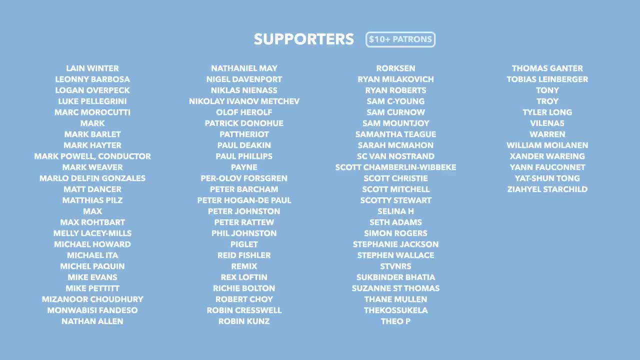 description: Thanks for watching and we'll see you in the next one.